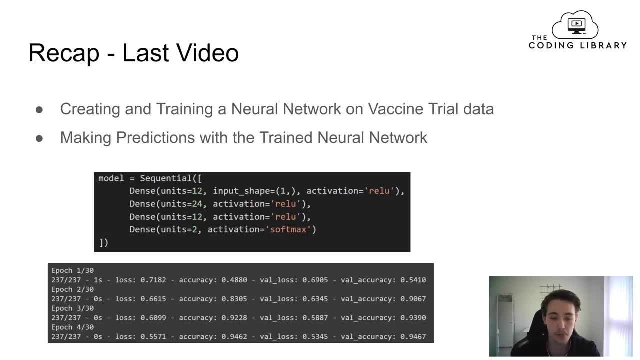 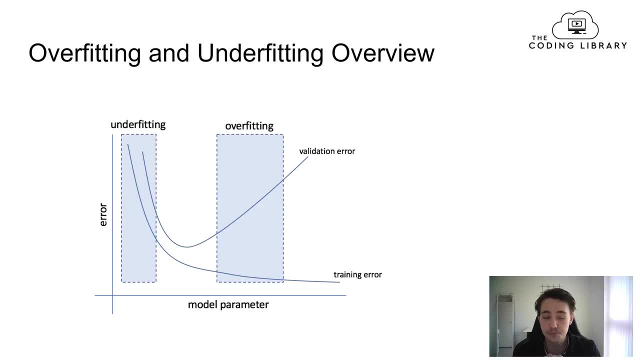 that we did and made predictions on the trained neural network. So in this video here we're going to talk about overfitting and unfitting And first of all, I want to give you an overview over what it is And I have this graph here, or like this figure here to like show you what overfitting and unfitting is when we're talking about like a trained neural network. So we have this error up here, So we want to decrease our error when we're training a neural network. So we can see that these two errors, or like these two lines of graphs here, is going to be. 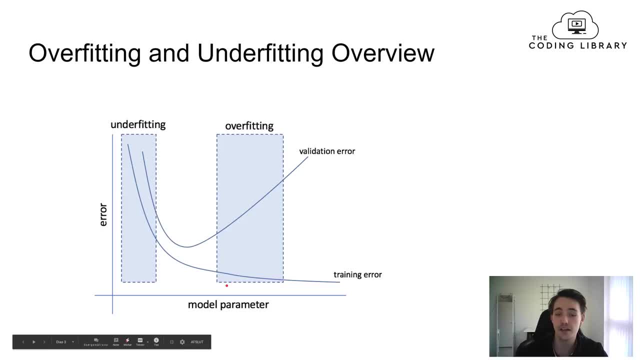 going down And then we have the model parameters down here. So we want to find, like the model parameters, which has like the best loss rate or like the error rate, So we don't have error when we're doing new predictions with our neural network. So first of all here we can see that these two graphs here they're following a pretty good along here where we have in this unfitting area. So first of all here, when we haven't trained our neural network that much and we have these model parameters here, then we can see that our model is unfitting So we can't do predictions on new data because 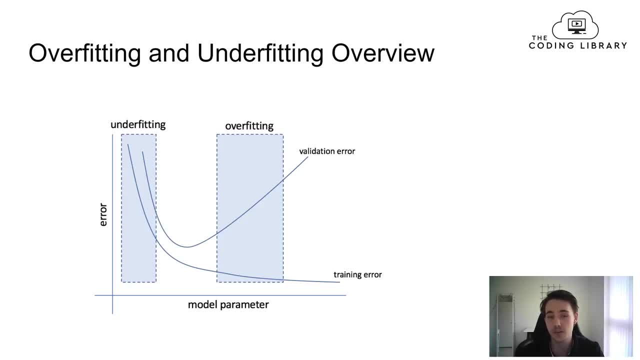 our neural network is not able to like generalize and do new predictions on what we wanted it to. So that could be caused by some different kind of things like not enough complexity in our neural network or not enough training data that it can learn from. So we're going to talk about that more in depth here in this video here as well. So we can see that these two graphs here they're following pretty good along. and then we have these model parameters. So at one point the model parameters here we can find like the optimal model parameters for this neural network here. 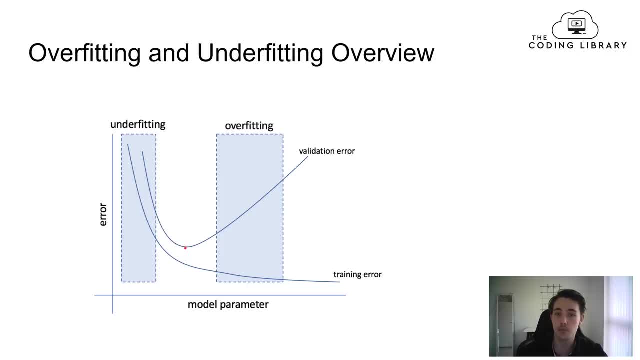 When it's training. and then we can stop at when we hit these model parameters here with our neural network, because when we hit these model parameters here we can see that our validation error starts to go up and we start to go up in this overfitting area here and the like. the objective of training a neural network is to get the loss towards zero, or like converge towards zero, or like at least close to zero. So because we don't want errors when we're trying to do new predictions with a new neural network on data that our neural network hasn't seen, 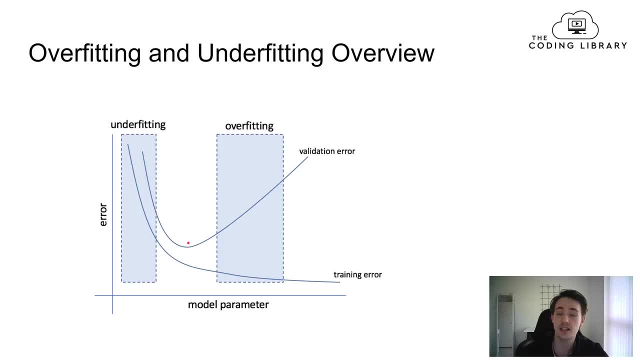 Before. so we can see here like if we train it too much or like our model is going to overfit, we can see that the validation error here it goes up and it it just goes further away from the training error. So the objectives here is that we have a training error here. that can be pretty good. But if our validation error is not a good and far away from training error, then our neural network is overfitting, which means that we have overfit our neural network to the data that we have trained it on and it is not able to do predictions on data that it hasn't seen before. 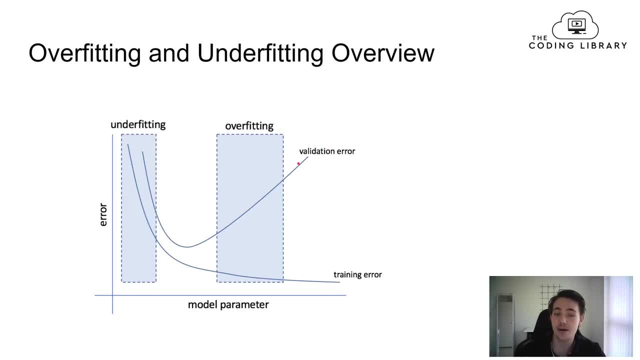 Because we like, we can't validate our model and we will get a high error when we're trying to to to do new predictions on data that it hasn't seen before. But we can do fine predictions with, with the, with the like, the data that it has trained on, but our model has just overfit and so we can't like, we can't like generalize and generalize our model so we can do new predictions on new data. So this is very, not a- very important features and very, very important things in neural networks when we're training, and some of the most important ones is overfitting and underfitting. 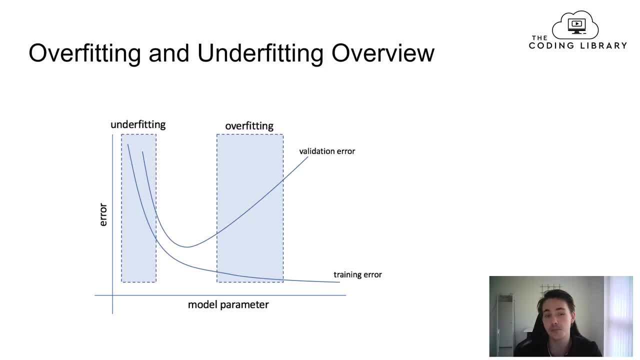 And these, these are like very things, like very important things to to keep track on and like know what happens when you're training a neural network and also how to how to reduce overfitting and underfitting, because these are the most like common errors when you're training a neural network. 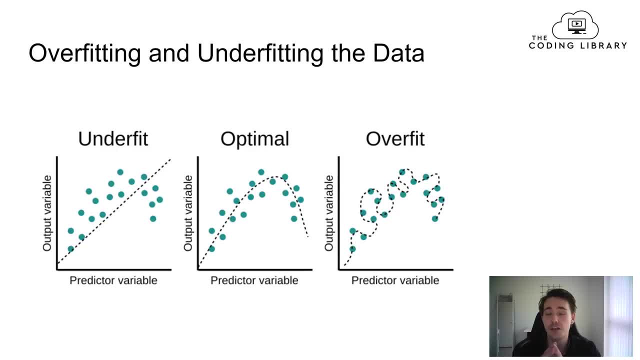 So first of all, here we're going to see, like, what is really like overfitting and underfitting the data in a neural network. So we can see over here if we, if our data, like, if our model, is underfitting here, we can see that we have a predicted variable here and then up here on the white line. 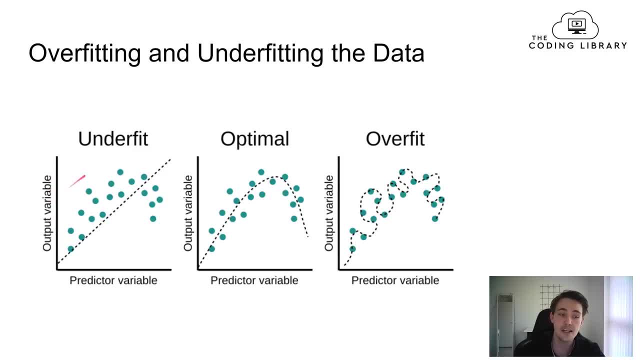 We have the output variable that we're going to predict with a new network and we can see that if we have an, an model here that is underfitting, then we're not really good like we can't really like predict the new data because our model is not in a complex not so we can't really predict what we wanted to. 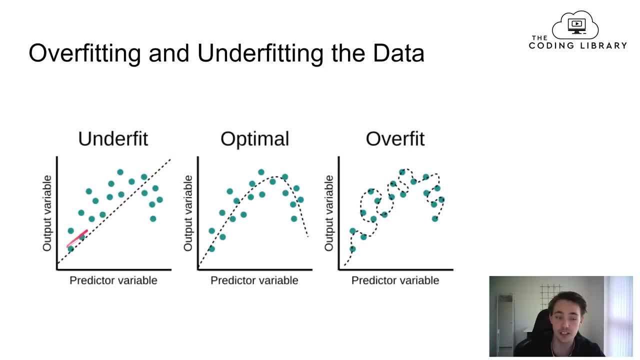 And we can see here that we have this optimal here. so here we just have like a straight line here, like linear regression for example, and we can see that we have these different kind of predictions here and they're really far away from like um, from like a model or like our regression line here. but the more optimal one here would be like: 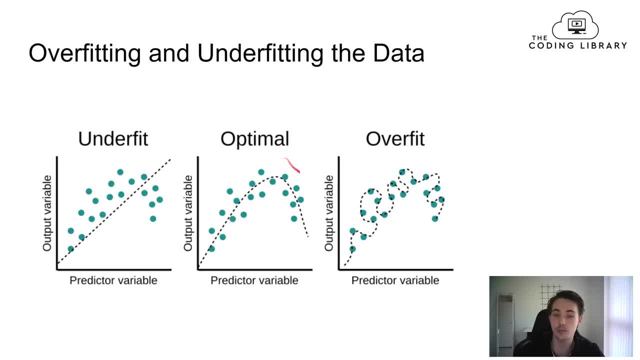 um, where we have this like kind of regression here that goes through all the points and is pretty close to it and we can still generalize our data and- and we're not overfitting on the data- we can see that we still get get some deviation from uh, from like optimal or like. 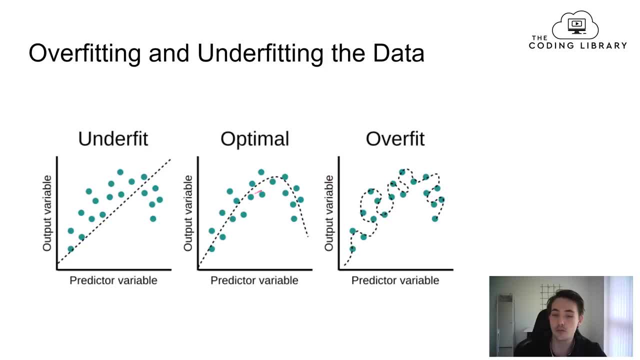 or from our regression line on this neural network here and then over here to the right, we have this overfitting scenario where our model is just overfitting so much to the overfitting, so much to the data that we're training on, that is not able to predict. 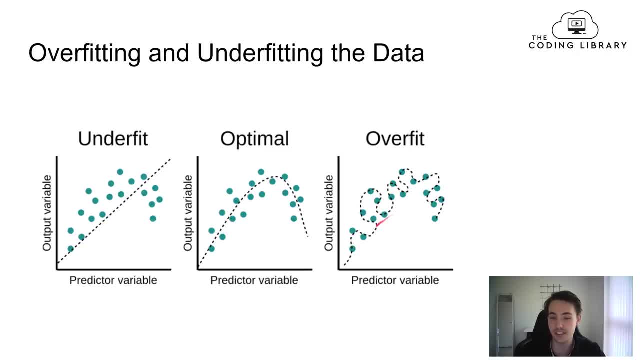 um to predict a new data that it hasn't seen before. so we can see that we get this very, very complex output and this overfit here of the data. so we can see that it's try, it tries to fit to all the data points instead of making making it generalize a bit where we can see this optimal. 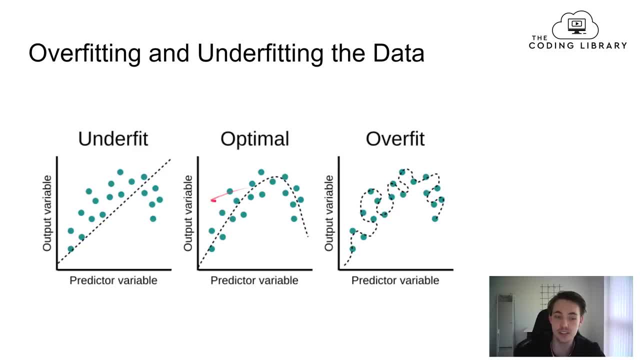 solution here: like we can predict new data variables. like we can see that if we do new predictions here, like we will get new points down here, where up on this graph here, if we did new predictions, like we will get a values up here where we wanted to get them down here. so we have this optimal solution. 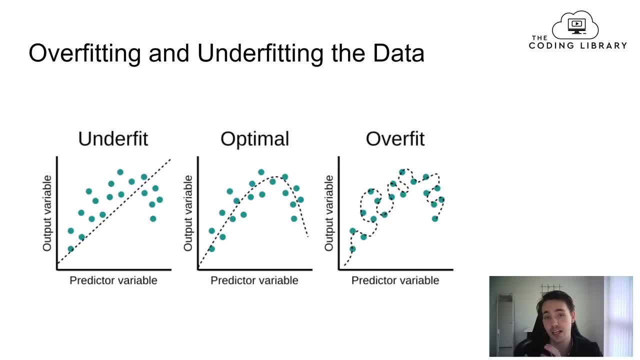 here, um, where we're not underfitting, we're not overfitting and we can have new data and predict, uh, and do predictions on new data that our neural network hasn't seen before, and over here on the overfitting, we won't be able to do actual new predictions with. 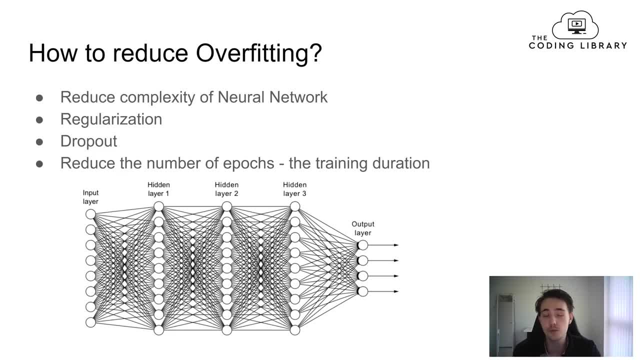 data that it hasn't seen before. so how can we reduce overfitting? if our neural network is overfitting, uh, when training it? so first of all, we can start with trying to reduce overfitting if we have a really, really complex neural network. so if you have a really really 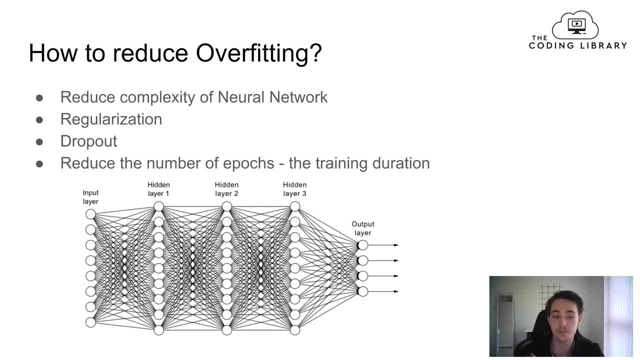 complex neural network and we're not really doing a complex task, then we can reduce some of the complexity by probably taking out some of the hidden layers- if we have too many hidden layers- and also trying to take out some of the neurons in um in some of the layers and see if that reduces. 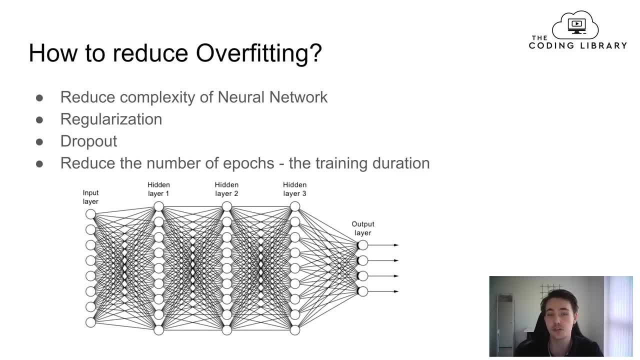 overfitting when we're training on your network again, we can also use something called regularization, which we're going to cover in in another video, because it's a really cool and nice feature so we can play around with some of the different kind of like parameters and activations. 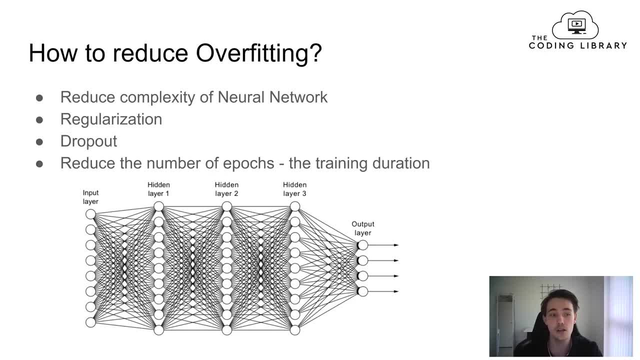 that we have in our neural network with regularization, so it's really cool and nice uh features. so remember to subscribe. hit the bell notification as well, so you will get a notification when i upload a video about regularization in this in deep learning tutorial we can also use. 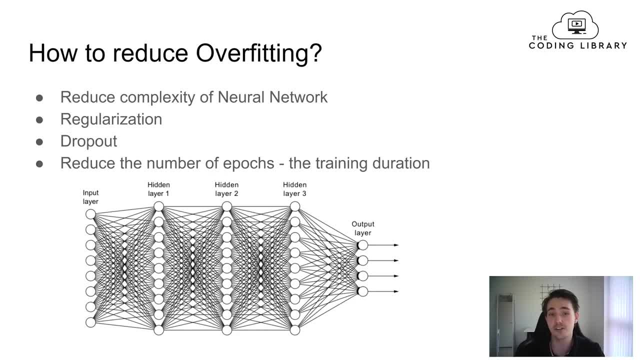 something called drop art, where we're just having- we can have dropout layers or dropout neurons. so when we're training a neural network we will just drop out some of the neurons. so we reduce the complexity of a neural network and we can also reduce the number of epochs, so the number like 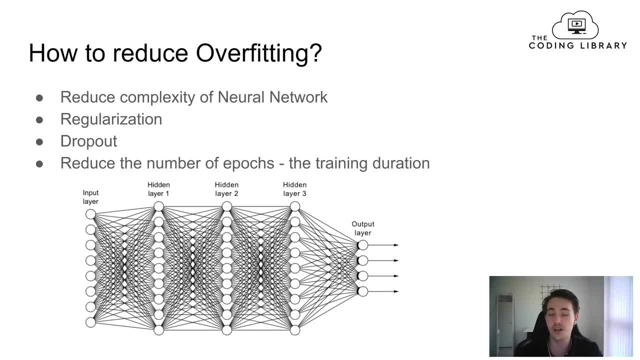 so we don't train for that long, as i showed you on the first graph with the overview. then we can stop the training process when we hit the most optimal parameters before our validation loss starts to increase again, because we want it to decrease and be kind of the same as our loss. 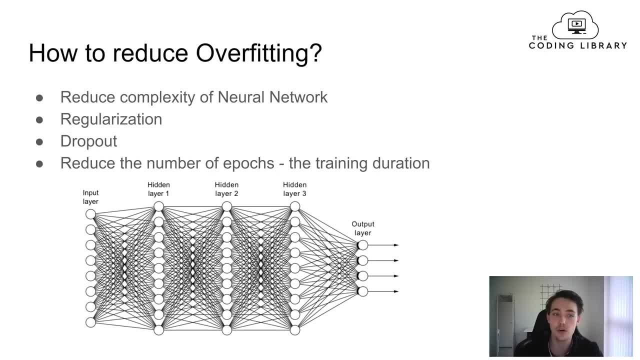 or as our training, training error. so this is a way to overduce overfitting and it's it's really nice and we're going to cover this more in other videos. but you can try out with reducing the complexity and using some of these methods here for regularization. so if you want to, 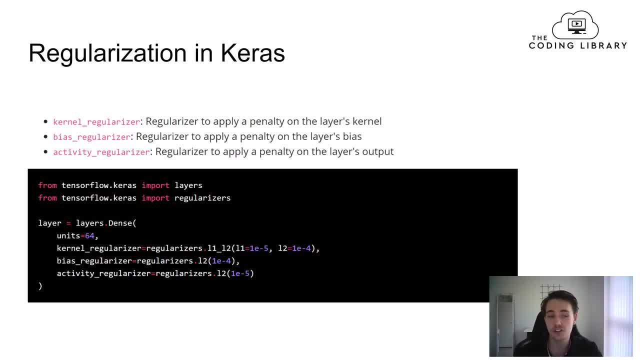 do this regularization here in carriers. there's some building functions where you can just apply it. we're going to cover some l1 and l2 regularization and some other different kind of methods, but this is just like how, if you want to do it in carriers where you can import these. 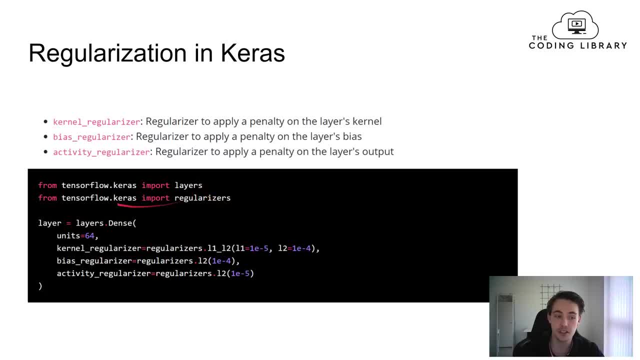 regularizations, regularizers here from the tens flow carriers, and then you can just specify in your layers like what type of what, if what type of uh regularization you want to use um in a layer in your neural network, and then it will do um, and then it will do all that with 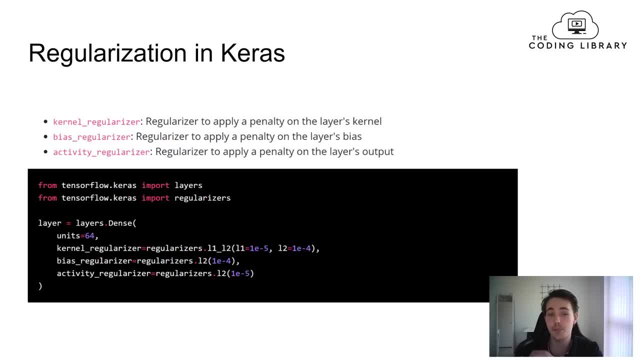 training and where you're training your needle network, then they will use this to like panel penalize um the either, like the la, is a kernel or bias or the latest output. um, as you can see up here, we have some different kind of um regular rises for a kernel and the buyers and activate activity. 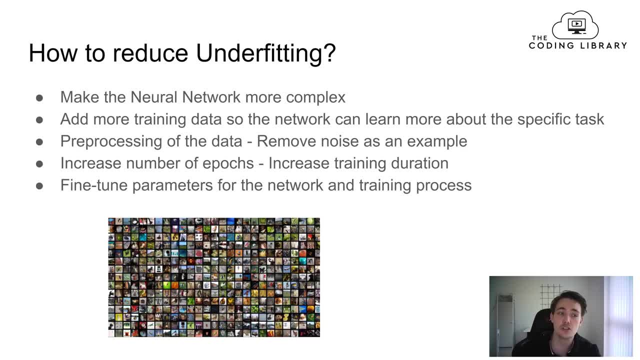 so the layers output. so if we have underfitting in our neural network when we're training it, we can reduce it some in some different kind of ways as well. so first of all we can start with making our neural network more complex, because Because when we're underfitting, our model is not generalizing and it's not really fitting. 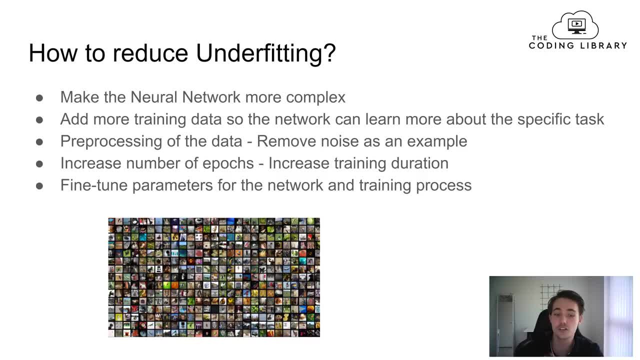 that good to our data, as we already saw. So we can't do predictions of what we want on new data because our model is underfitting and it's not really that complex. So we can start with adding, for example, layers or new units to our new network and 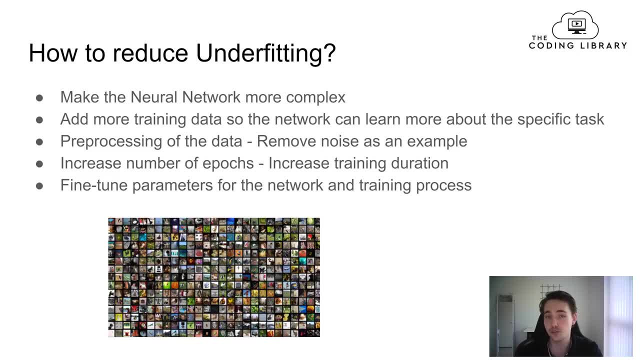 try that and see if we can reduce underfitting and we can actually do predictions on new data, Or we can either, like in some of the cases, in a lot of the different kinds of cases, we need to add more training data so the network can learn more about the specific task that 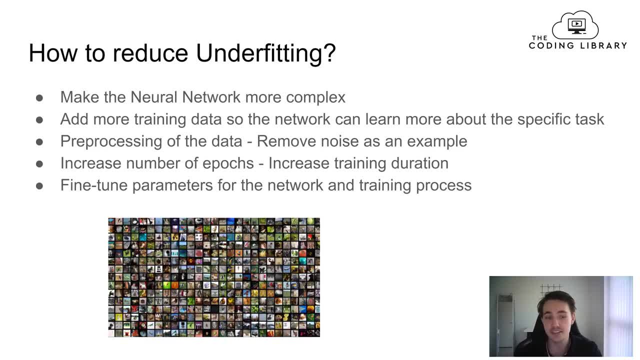 we're going to do, And it both applies for ANNs and CNNs. So often when you're having CNNs, you just want like, if your application or your neural network is underfitting and you can't predict new data, then it's probably because you don't. 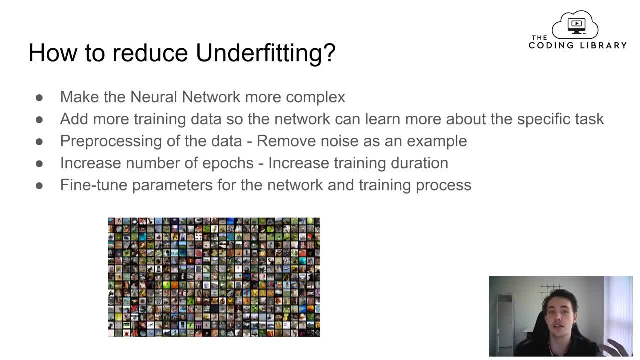 have enough images that your neural network can learn off in the training process, So you can start with adding more data to it And try to make it more specific. Try to make your model more complex to avoid this underfitting, or at least reduce the underfitting. 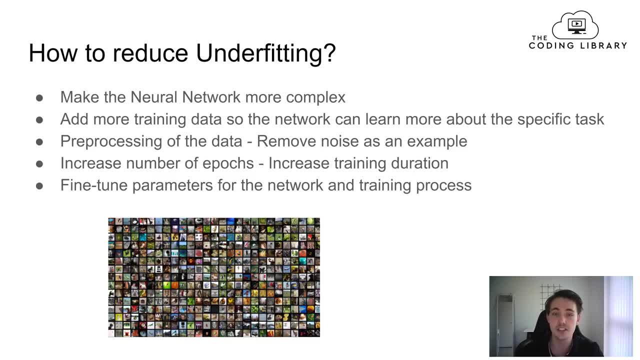 We can also do some pre-processing of the data, So, for example, we can remove the noise as an example and we can get more like we can get better and more precise data, And then we can use that data to make our model do more complex things and avoid underfitting. 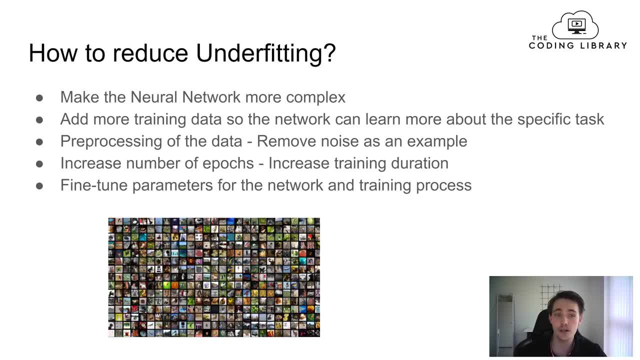 And we can also increase the number of epochs. So we increase the training duration where in overfitting we wanted to decrease the number of epochs. But if we're just training our neural networks more, and more and more, then we can also reduce some of the underfitting. 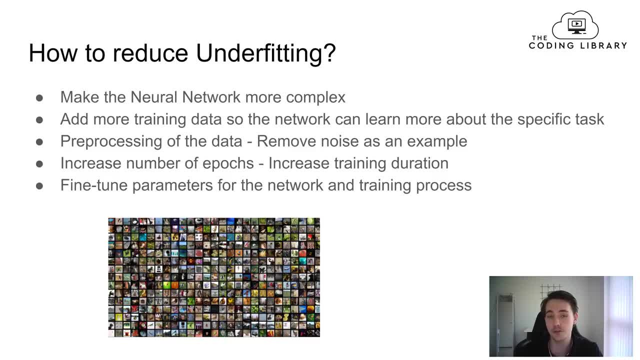 As we saw on the overview slide where we can see the model parameters, they can still go down if you just train our model for more epochs. But if we don't have enough data- and that's the cause of underfitting- then it won't really. 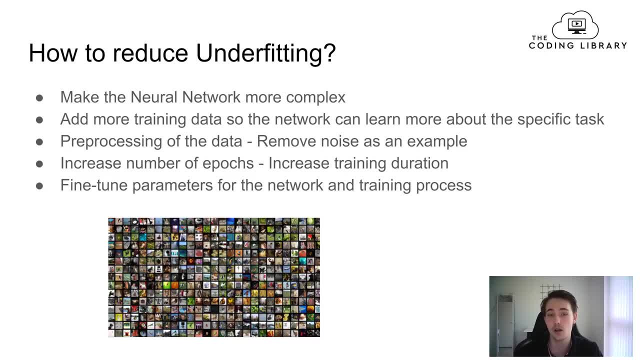 help to just increase the number of epochs. if the model that it's training on, if it needs more data, then it doesn't really matter of the number of epochs or if your neural network is not complex enough. So make sure to start with training. 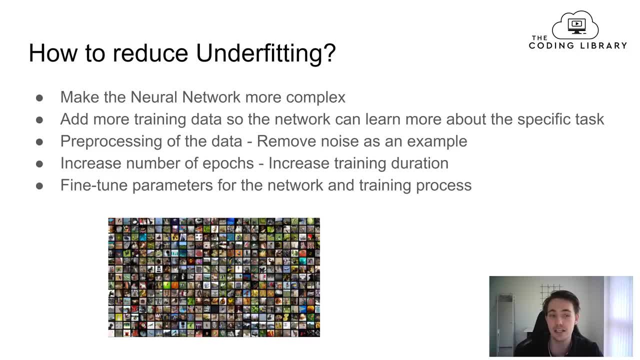 Starting out to make your neural network more complex and add more training data, And then afterwards, if that doesn't work yet, you can try to increase the number of epochs or pre-process- some of the data that you feed to the neural network when it's training. 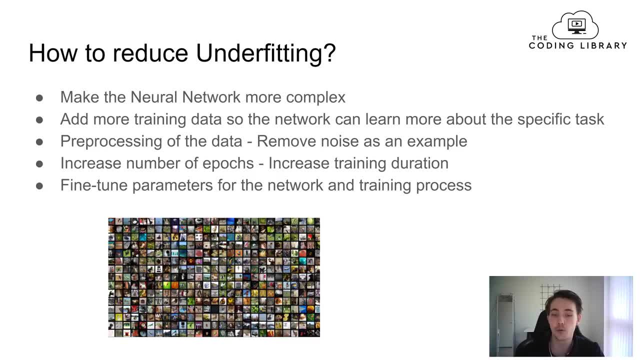 And the last option here is that we can fine tune some of the parameters for the network and training process with the learning rate and some of the different kind of parameters that we can fine tune- And we talked about those in some of the previous videos, so check those out if you don't know. 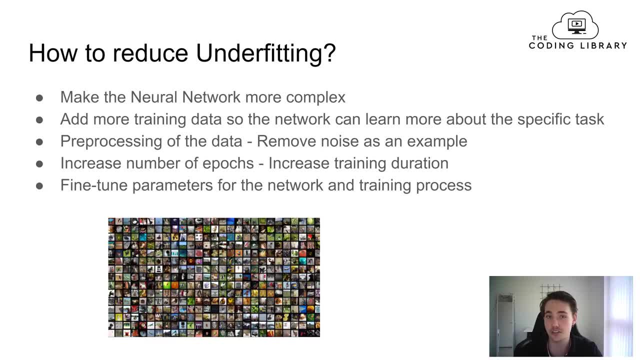 what different kind of parameters that you can tune in a neural network and in the training process of a neural network. So that's pretty much it for this video here, guys, where we know what is underfitting and overfitting in a neural network when we're training on a neural network. because these 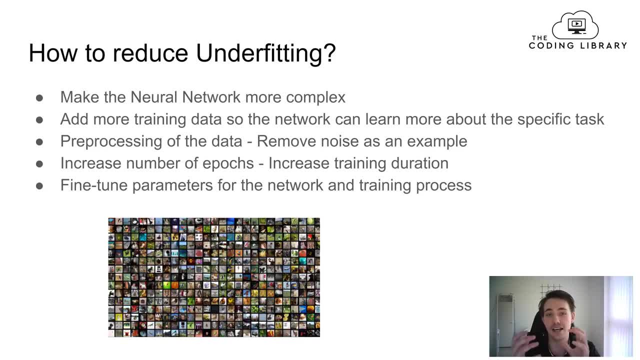 are some of the most common faults or errors in our neural network when we are training. So we don't want our neural network to underfit or underfit and overfit and we want to find some nice balance where we find the most optimal model parameters for a neural network. so we 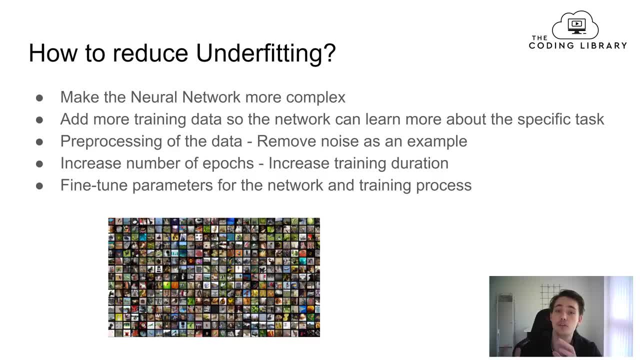 can generalize good on new data and we're still able to actually predict a new data that we want to predict And we can. also, it doesn't just fit to the training data, so we can't predict a new data that the model hasn't seen and trained on before. 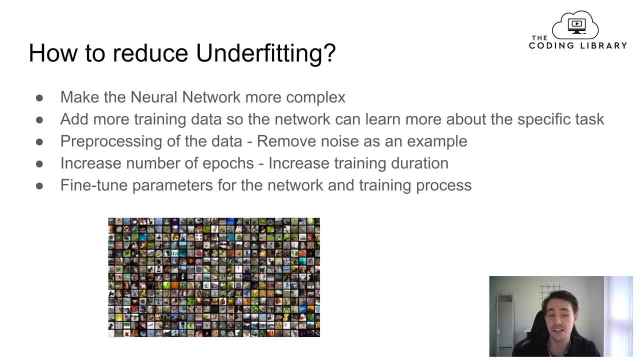 So these are very nice and very important things in neural networks and when we're training a neural network and also just how neural networks work in general. So thank you guys for watching this video and remember to subscribe button and bell if you haven't already. 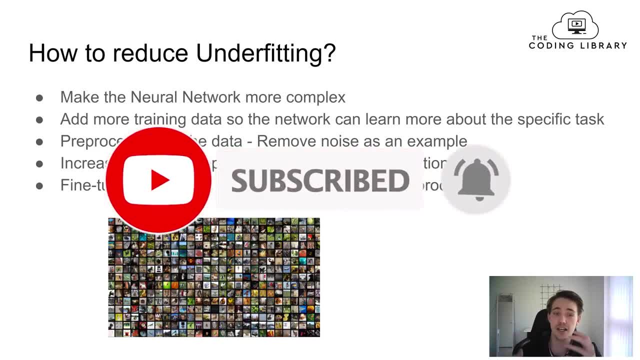 Like this video here, if you like the content and you want more in the future, because it just really helps me and the YouTube channel out in a massive way. So I really appreciate your support. and if you're interested in one of the other tutorials I'm doing, I'm also currently doing a computer vision tutorial in C++ and OpenCV and an algorithm. 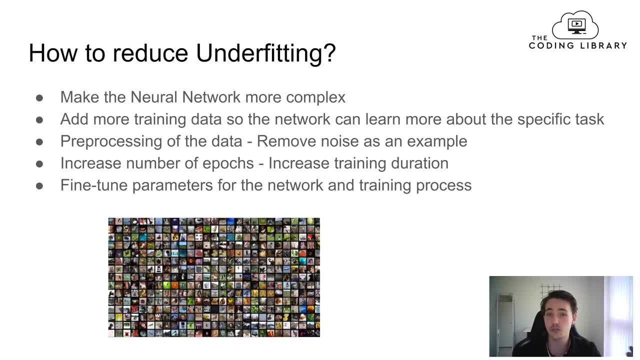 data structure tutorial in C++ as well. So if you're interested in one of those tutorials with computer vision- and we're also talking about computer vision and deep learning together and how they work together and how we can use that- So if you're interested in one of the tutorials, I'll link to one of the tutorials in the description. below. I'll put a link to one of them up here, or else I'll just see you in the next video, guys. Bye for now.